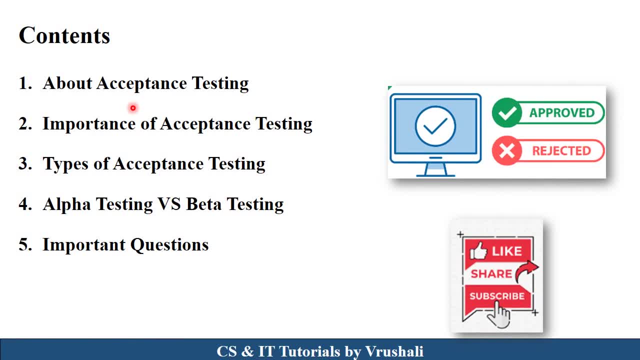 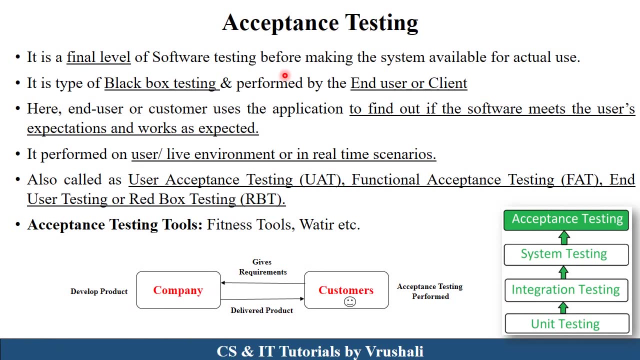 start the session. In this session we will discuss about acceptance testing, their importance types, alpha versus beta testing and some important questions that have asked in previous year question paper. Let's see all these points one by one Now. the first topic is: what exactly? 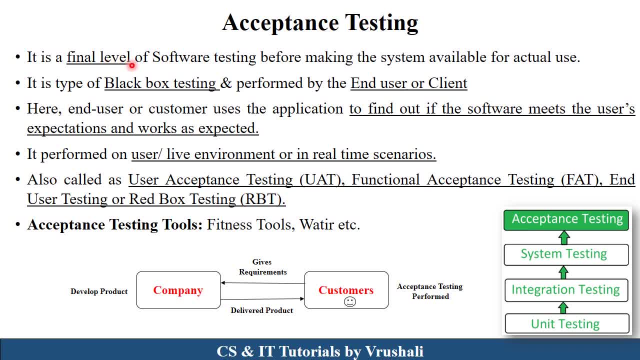 acceptance testing. Acceptance testing is final level of testing in software testing process. See here in this particular image. We already discussed unit integration system testing in previous session. In unit testing tester test each and every modules components mentioned in your project individually. In integration testing tester test a complete. 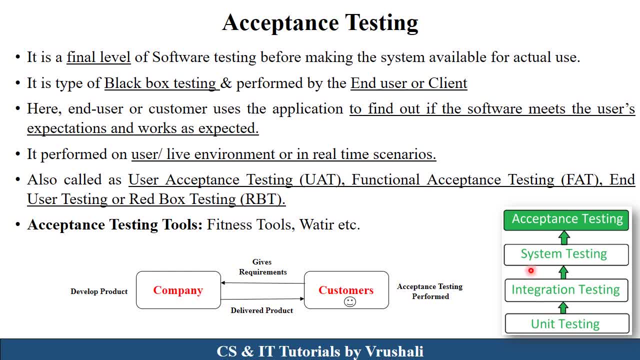 product or a project at a same time, In system testing, tester test a overall behavior, functionality, accuracy and quality of your product. And now there is acceptance testing. See here, in this particular image, There are some IT or software companies and there are some 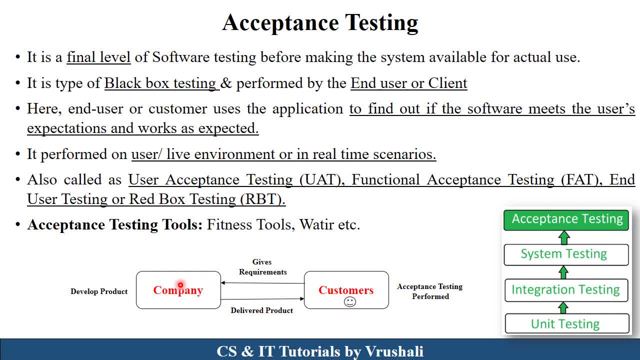 customers. customer gives a requirements to the particular company. company develop a product as per the customer requirements. now after developing, company delivered a product to the customers. now at customer side, customer test that a particular product a develop as per the customer requirement, customer expectation and customer need. so this is called as acceptance. 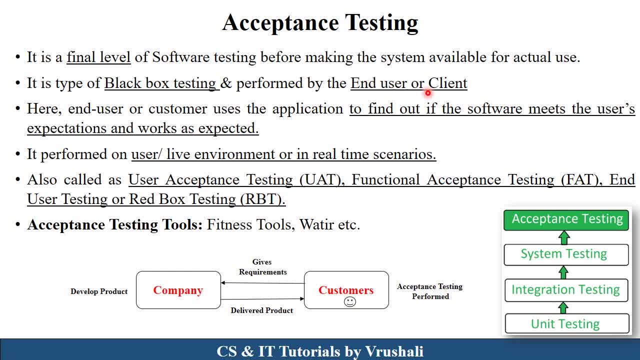 testing. acceptance testing perform by the end user or client, where customer test a particular product with real users and in real life environment. acceptance testing is a type of black box testing because they mainly focus on expected output of particular product. acceptance testing, also called as user acceptance testing, functional acceptance tasting a شيse testing- 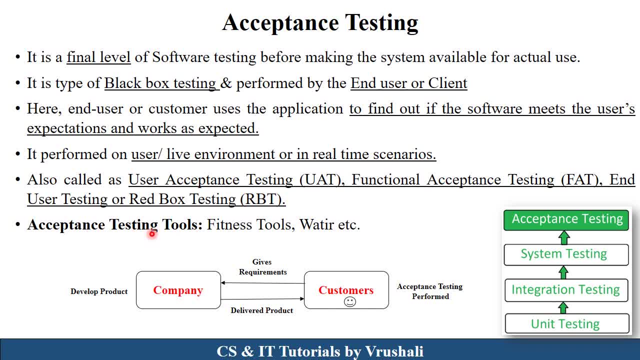 or red box testing. There are different R vita types of acceptance testing and we will be discussing the colors names jadi In todays separate ajewith the American market, the safety. we are work in the area of marketing. different acceptance testing tools are available in market. 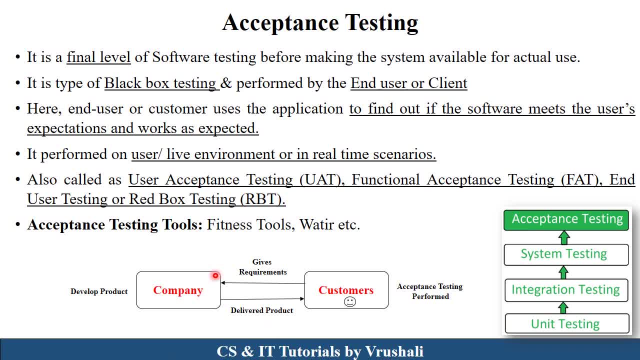 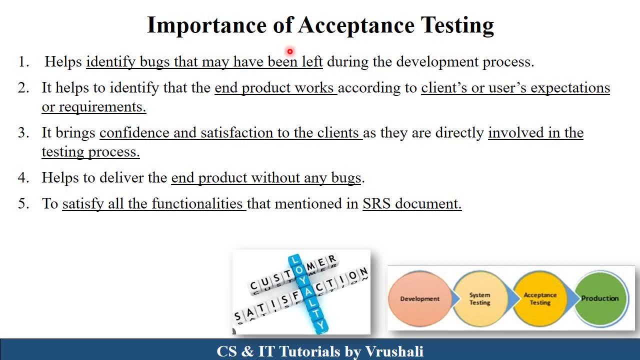 So, basically, unit integration system. this testing are performed at company site or by the developer or tester, and acceptance testing perform at customer site. Now the next topic is importance of acceptance testing. due to acceptance testing, they identify all the bugs or errors that may have been left during development process. 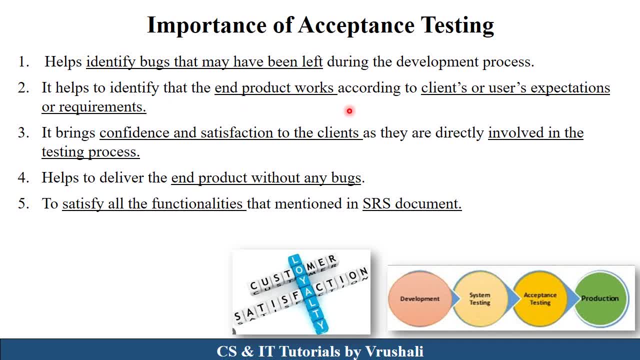 They identify that, whether a particular product developed as per the customer expectation or requirements, Acceptance testing bring confidence and satisfaction to the clients because customers are directly involved in testing process. Acceptance testing also ensure that to deliver a product to the end user without any bugs. 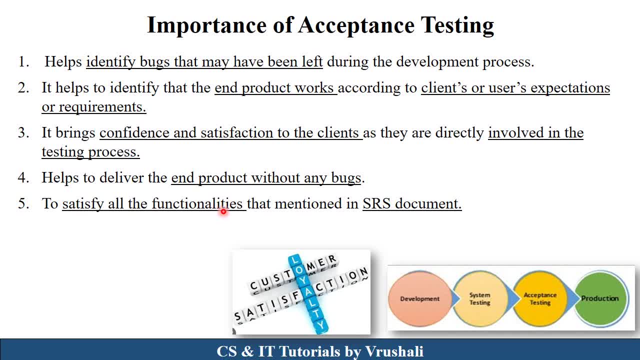 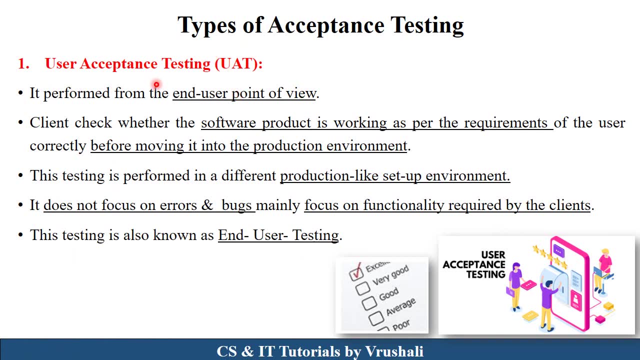 or errors. Basically, they satisfy all the functionalities mentioned in SRS documents. The main aim of acceptance testing is Customer satisfaction. Now there are different types of acceptance testing. The first type is user acceptance testing. User acceptance testing perform as per the customer point of view or user point of view. 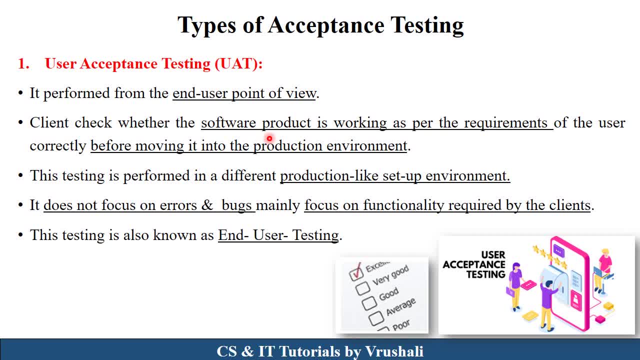 Here customer check that whether a particular software or product is developed as per the customer requirements, acceptation or need of the customer. After testing, then only product release in market. Customer acceptance testing perform as per the customer point of view or user point of view. 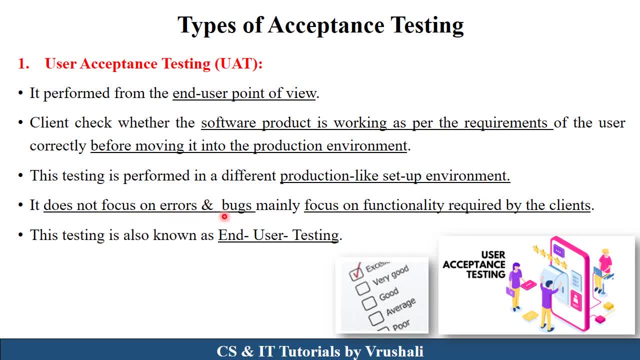 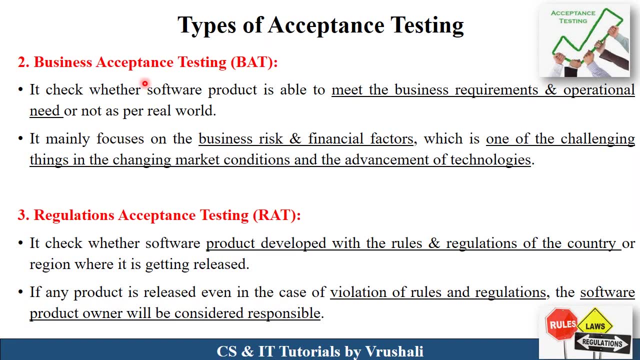 Here customer does not focus on errors or bugs in particular product. They mainly focus on functionalities or usefulness of particular product. This testing also called as end user testing. Now the next type of testing is business acceptance testing. See, there are some particular product have developed as per the business need right. 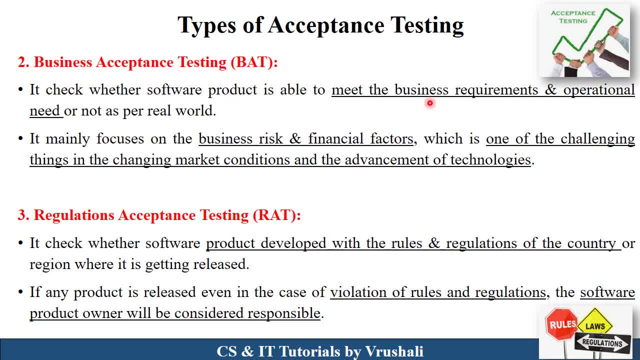 So here that customer check that A particular product meet the business requirement or operational need. We know that nowadays market conditions are continuously changing. right, There are different new technologies, new framework and new libraries are there right, So that particular product is developed or useful in that particular business need. 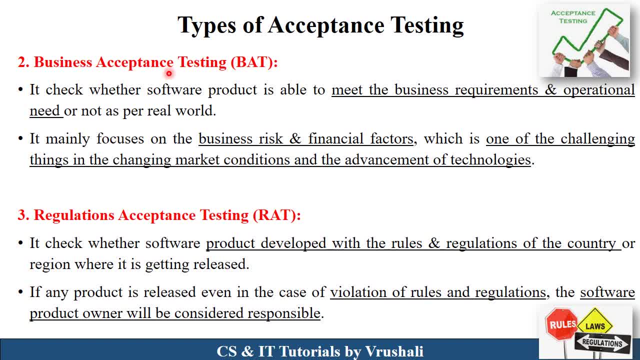 This all conditions have checked in business acceptance testing. Now the next one is a regulation acceptance testing. See In RAT tester. check that whether a particular software product is developed as per the rules and regulation mentioned by country or particular government. If a particular product violate rules and regulation mentioned by country or government. 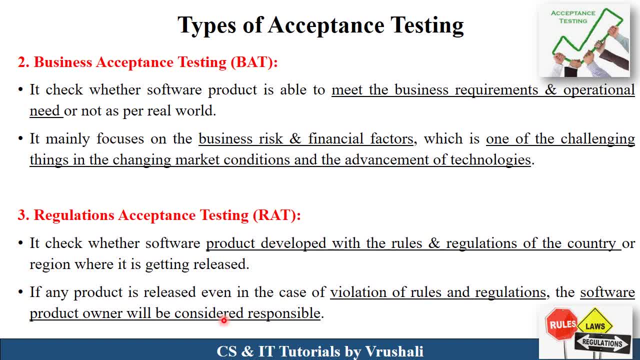 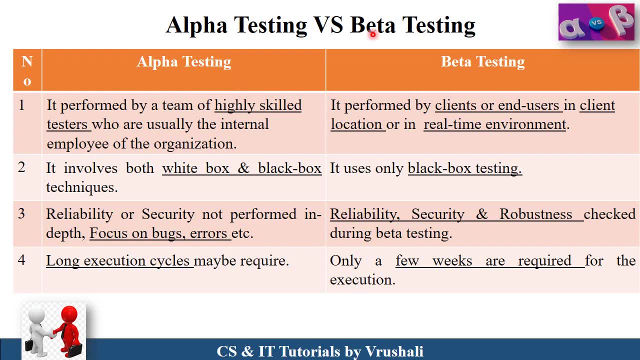 then software product owner will be considered responsible. So always develop a product as per the rules and regulation mentioned by the country or particular government. Now The next type of acceptance testing is alpha testing and beta testing. As per your exam point of view, this is one of the most important question. 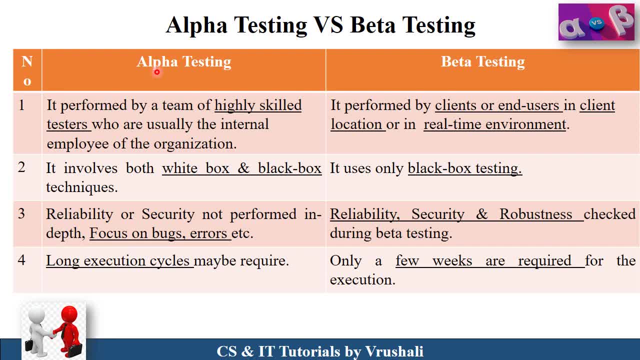 So here we will discuss alpha versus beta testing. Now see here: alpha testing is performed by highly skilled tester. This testing perform within an organization in testing phase of software development lifecycle. Beta testing perform at client side or end user side, And they perform with client side. 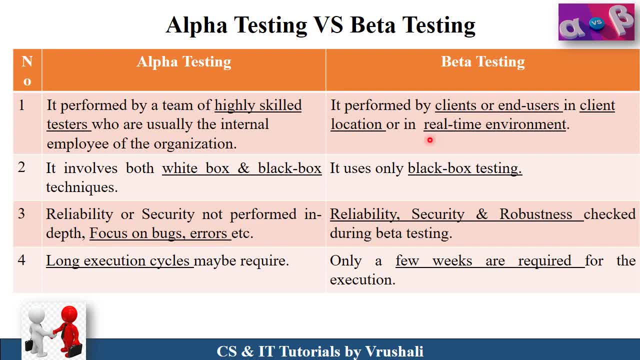 And they perform with client side And they perform with client location in real time environment with real users. Alpha testing involve both white box and black box testing. They mainly test complete internal structure, internal working and expected output of particular product. In beta testing, they only focus on expected output as per the customer requirement. 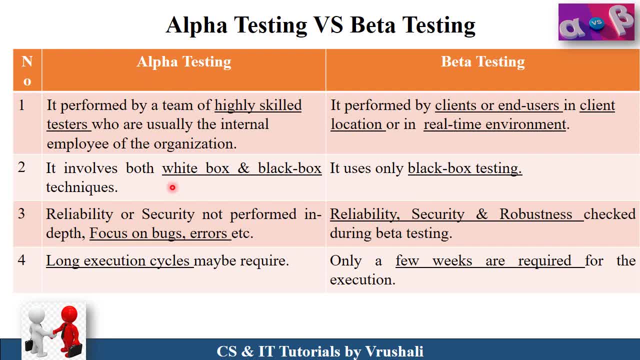 Alpha testing is a last testing of particular software development lifecycle testing process. Ok, After that it delivered to the customer than beta testing is performed. Alpha testing mainly focus on all the bugs and errors in particular product, But beta testing focus on reliability, security, robustness, accuracy of particular product. 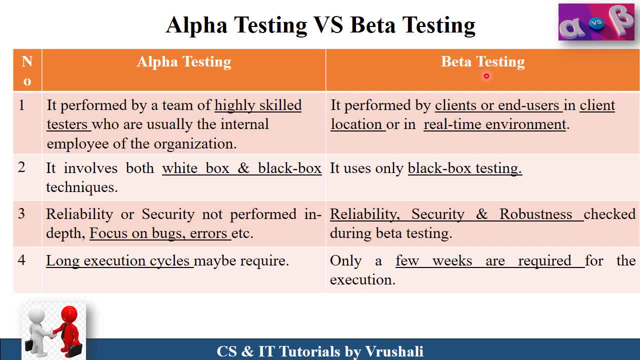 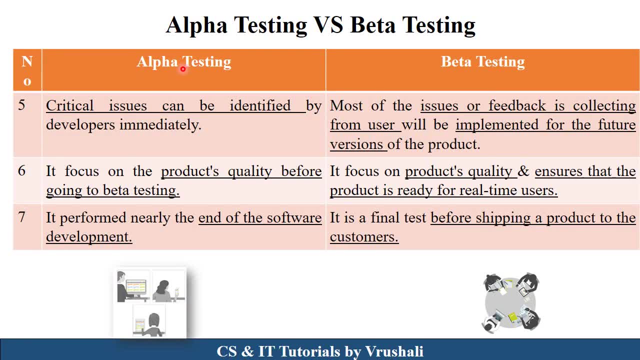 Alpha testing required long execution cycle But beta testing perform in few weeks as per the customer environment. Now in alpha testing there are some critical issues can be identified by the developers, So they solve all these issues immediately. But in beta testing suppose there are some issues or feedback from the customers are there. 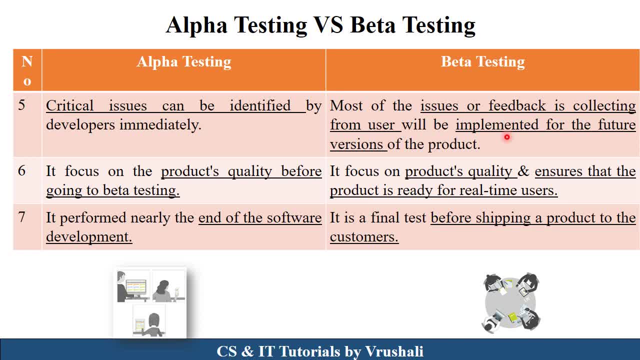 Now all these feedbacks are implemented in future version of particular product, which is called as beta version. In alpha testing it focus on product quality before going to beta testing, But in beta testing a focus on product quality as well as product is useful for real time users or not.